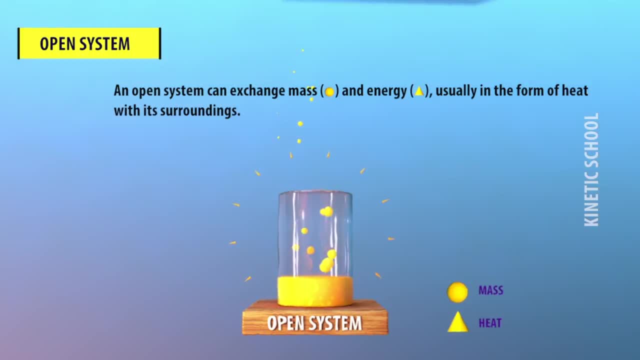 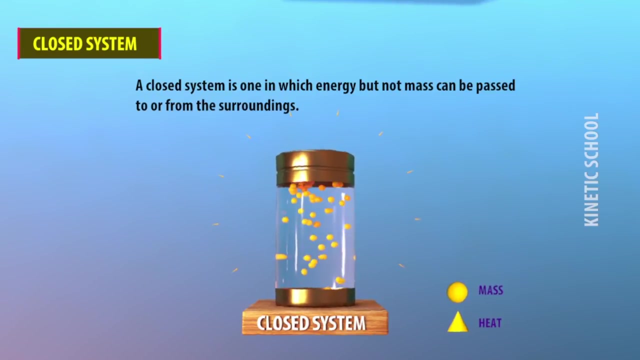 An open system can exchange mass and energy, usually in the form of heat, with its surroundings. Closed system- A closed system is one in which energy but not mass can be passed to energy but not air. A closed system is one in which energy but not air- A closed system can be. 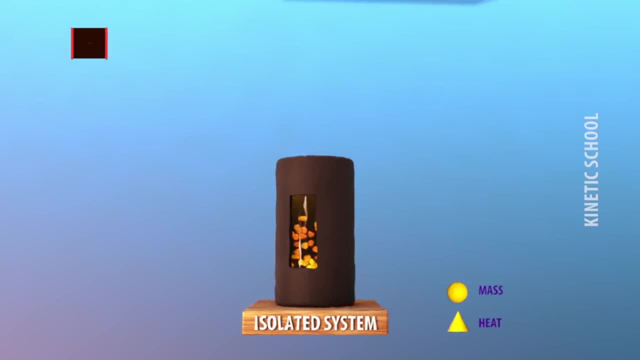 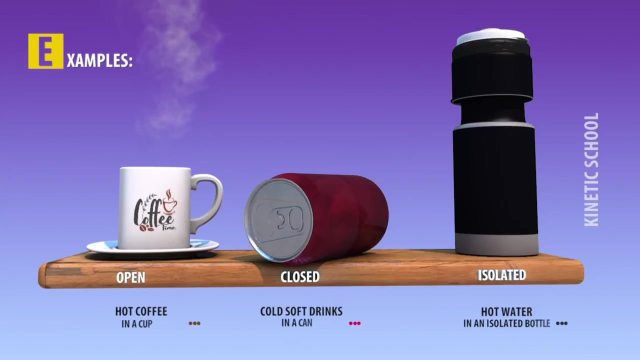 energy but not air. A closed system is one in which energy but not air. A closed system is one in op-touch or from the surroundings isolated system. an isolated system is one that can transfer neither mass nor energy to and from its surroundings. here are some examples of these three systems. 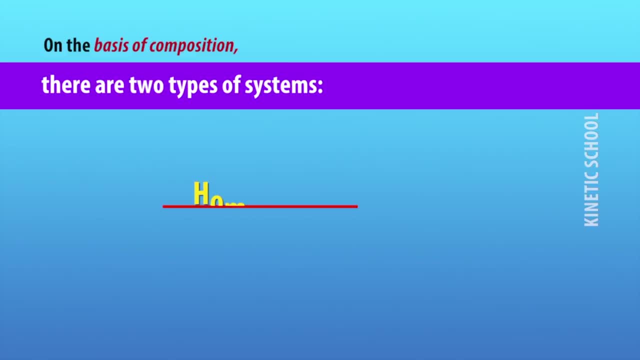 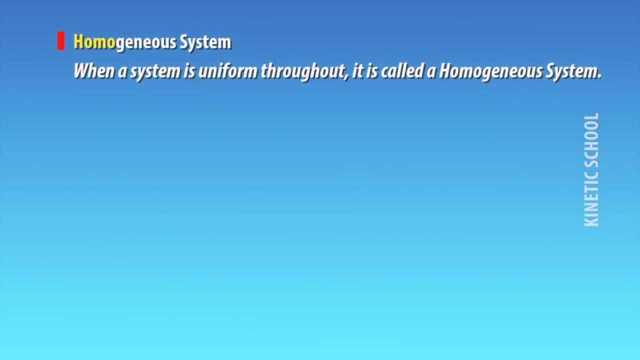 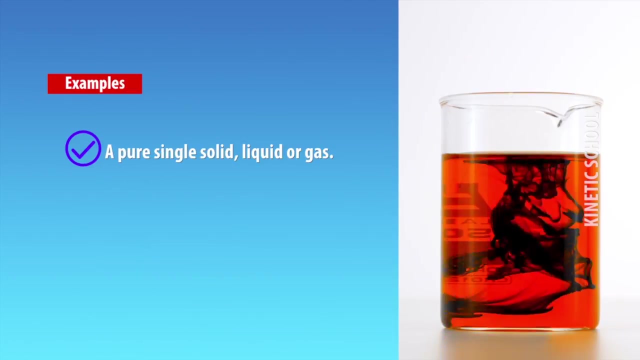 on the basis of composition, there are two types of systems: homogeneous system and heterogeneous system. homogeneous system: when a system is uniform throughout, it is called a homogeneous system. this system is made of one phase only. examples: a pure, single, solid liquid or a gas, a mixture of gases or liquids. such a system has one phase only. 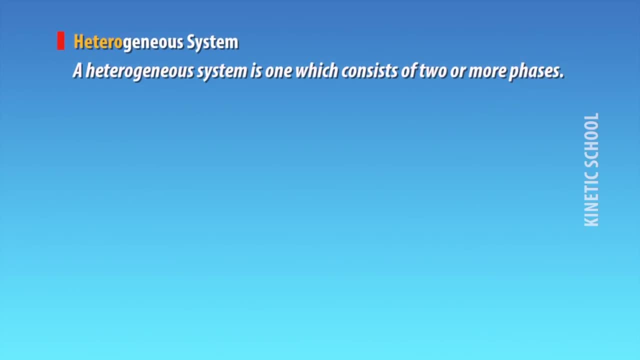 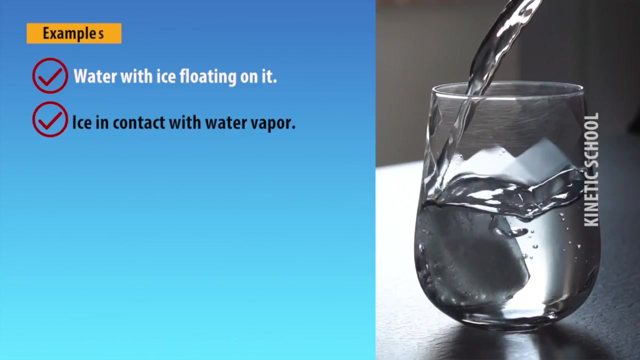 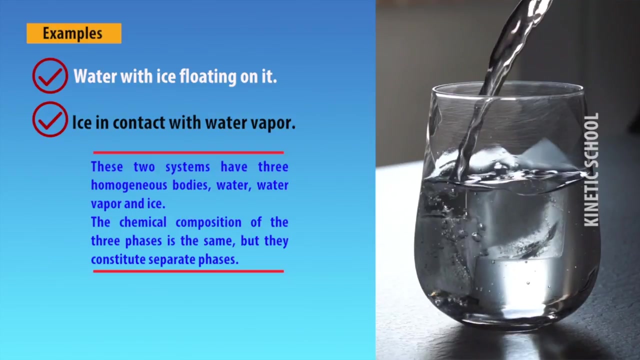 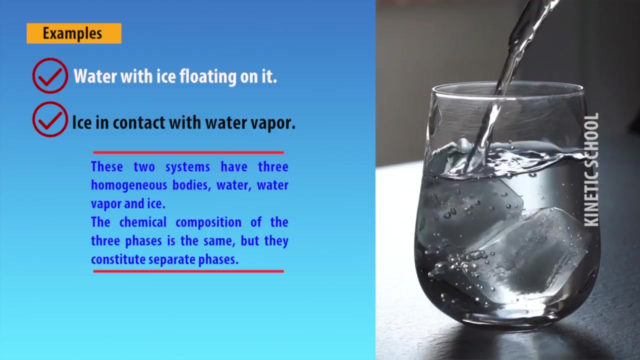 heterogeneous system. a heterogeneous system is one which consists of two or more phases. it is not uniform throughout. examples: water with ice floating on it, ice in contact with water vapor. these two systems have three homogeneous bodies, such as water, water vapor and ice. the chemical compositions of the three phases are same, but they constitute. 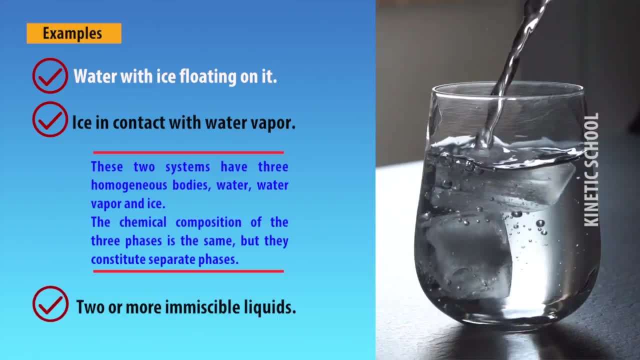 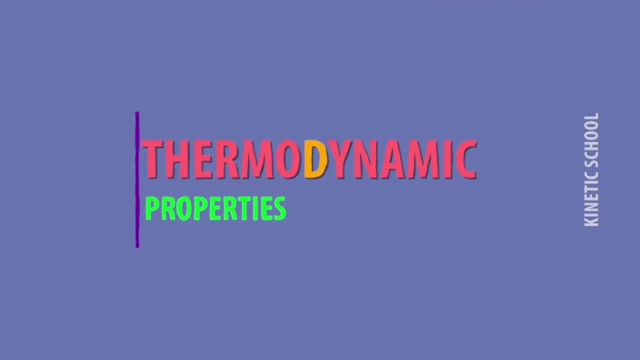 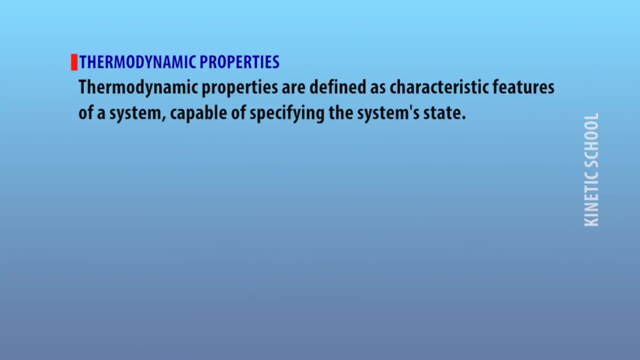 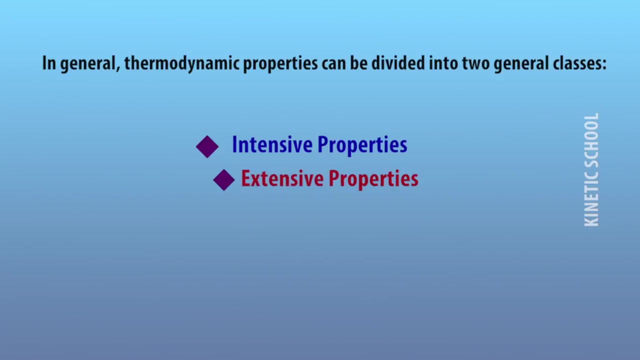 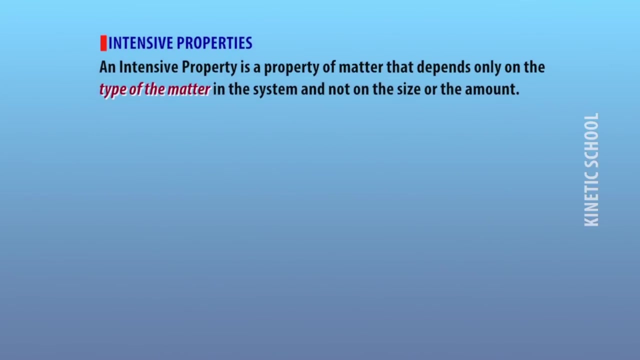 separate phases. one more example is two or more immiscible liquids: thermodynamic properties. thermodynamic properties are defined as characteristic feature of a system capable of specifying the system state. these are all microscopic in nature. in general, thermodynamic properties can be divided into two classes: thermodynamic properties and extensive properties. now, what are actually called intensive properties? 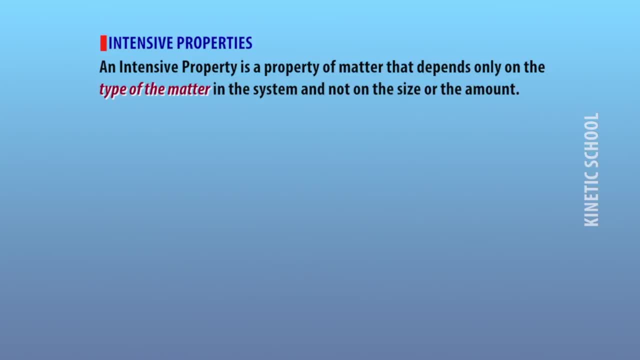 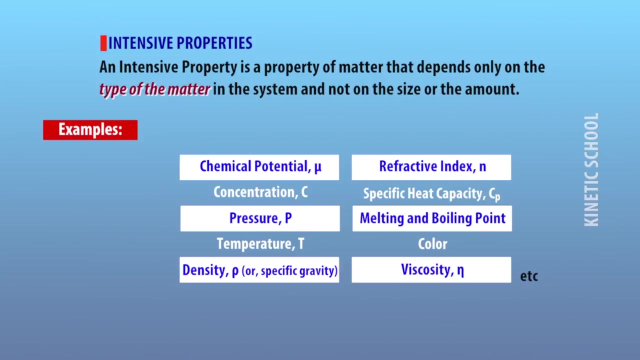 an intensive property is the property of matter. that depends only on the type of matter in the system and not on the size or the amount. for example, chemical potential, concentration, pressure, temperature density, Refraction index. Refraction index Specific heat capacity, melting and boiling point, color and viscosity. 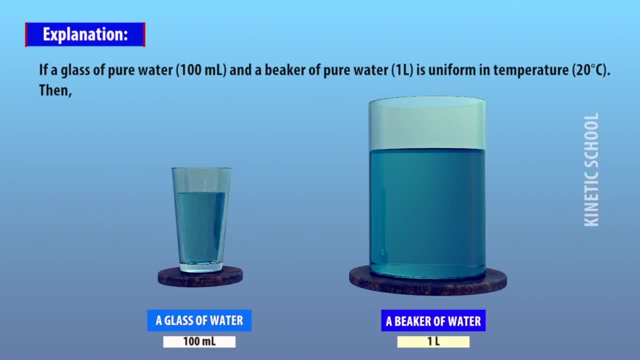 Explanation: If a glass of pure 100 ml water and a beaker of pure 1 liter water is uniform in temperature, which is 20 degree Celsius, then Concentration Density, Melting and boiling point, Reflective index, Color Viscosity, Specific heat capacity has to be same. 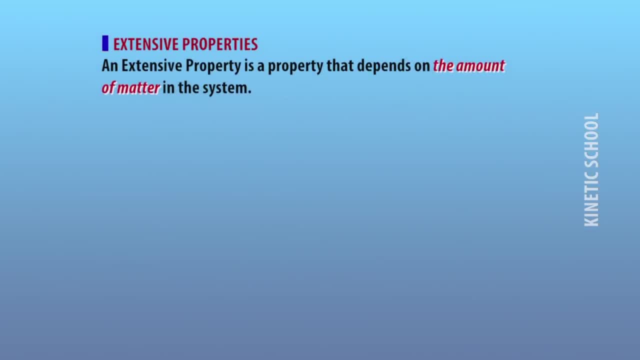 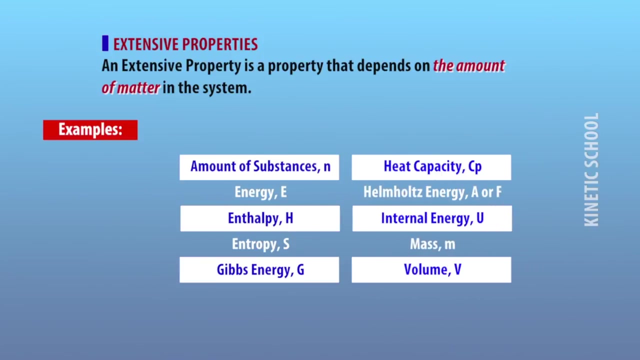 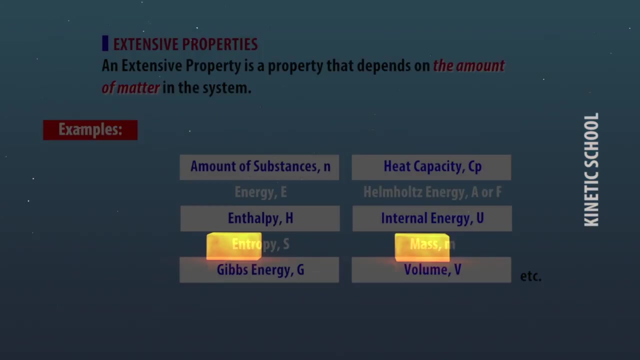 An extensive property is a property that depends on the amount of matter in the system, Such as Amount of substances, Energy Enthalpy, Entropy Gives energy, Heat capacity, Hemholes energy, Internal energy, Mass Volume. As we know, extensive properties are proportional to the amount of substances. 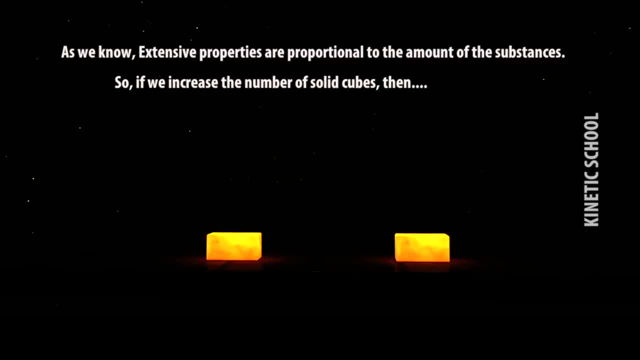 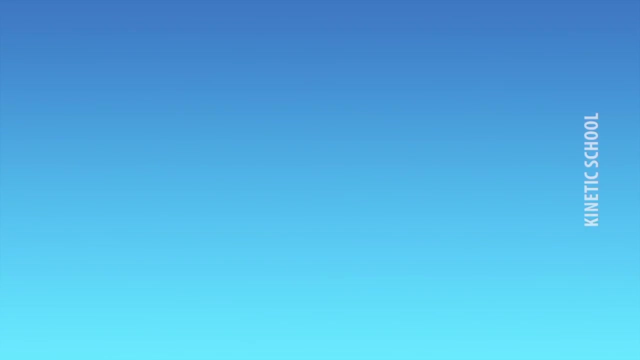 So if we increase the number of solid cubes, then Amount of substances, Mass Volume strategies, Heat Capacity, internal energy, enthalpy Energy has to be increased or decreased. State of a system: A thermodynamic state of a system is its condition at a specific time that is fully identified by the values of a suitable set of parameters known as state variable and physical parameters. 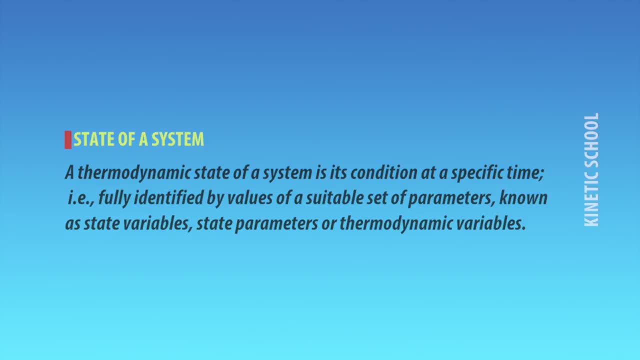 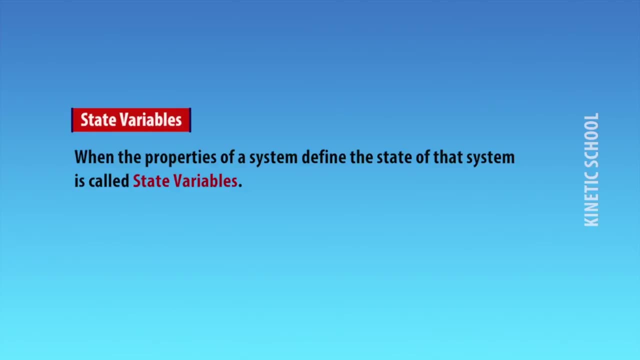 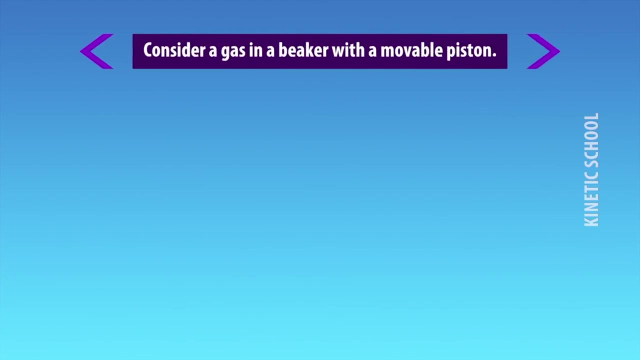 state parameters or thermodynamic variables. So how you define the state variables? When the properties of a system define the state of that system, is called state variables. Explanation: Consider a gas in a beaker with a movable piston. This is represented by state 1. 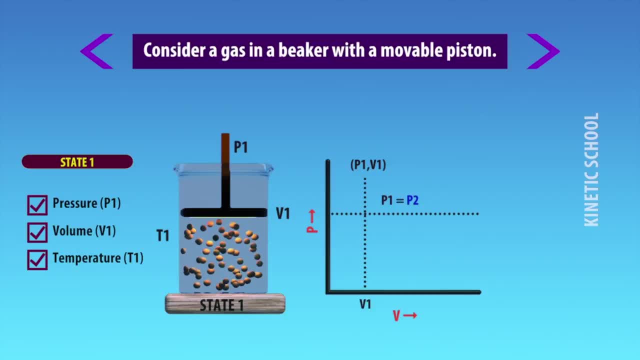 and it is having a fixed value of pressure, P1, volume, V1, temperature, T1, etc. Gas can be cooled or heated either in constant pressure or constant temperature or constant volume, etc. Then the gas is changed in another condition. The new condition is represented by state 2.. 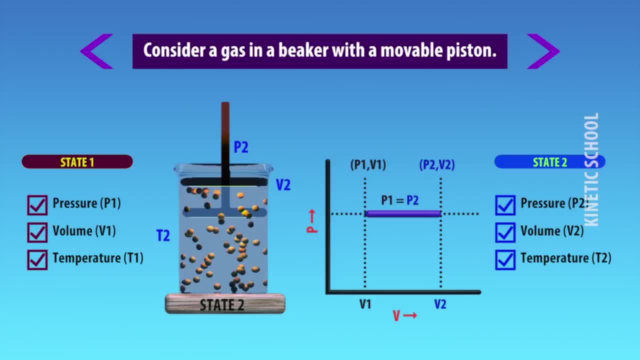 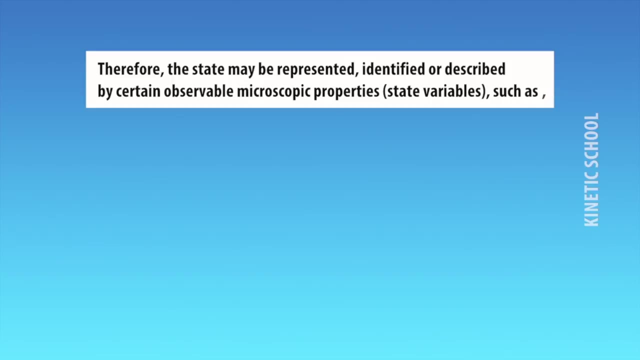 At state 2, it is having another fixed volume of pressure, P2 volume, V2, temperature, T2, etc. Therefore, the state may be represented, identified or described by certain observable microscopic properties such as volume, temperature, pressure, concentration, internal energy, enthalpy, etc. 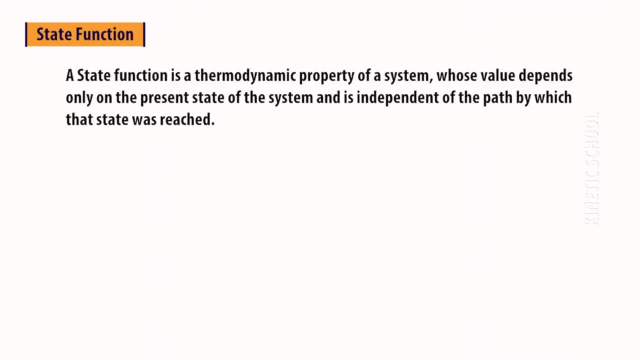 State function. A state function is a thermodynamic property. It is a state function. It is a state function. It is a state function. It is a property of a system whose value depends only on the present state of the system and is independent of the path by which the state was reached. 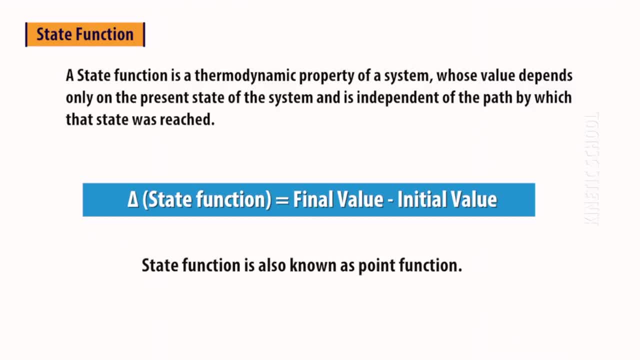 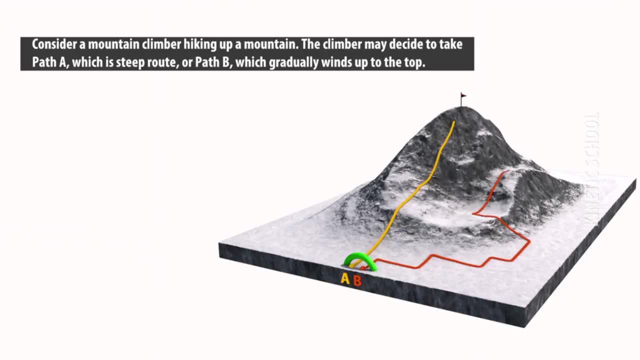 State function is also known as point function. Explanation: Consider a mountain climber hiking up a mountain. The climber may decide to take path A, which is steep route, or path B, which gradually winds up to the top. But climbing up by the direct route, which is path A, is more difficult, as it is almost vertical, than the curving route, which is path B. 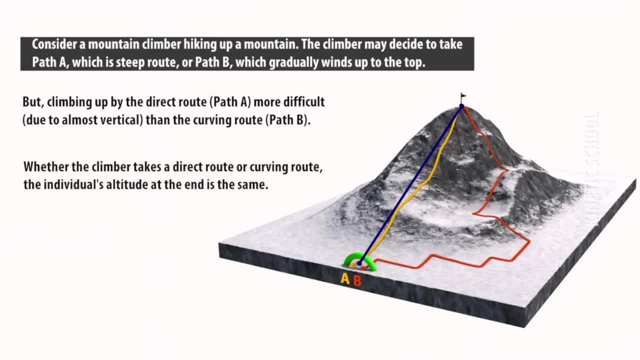 Whether the climber takes a direct route or curving route, the individual's altitude at the end is the same. Thus, altitude is the state function, because it depends only on the final destination, not how the climber got to that altitude. Similarly, 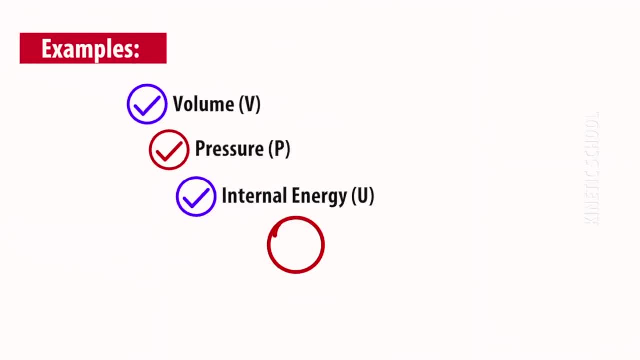 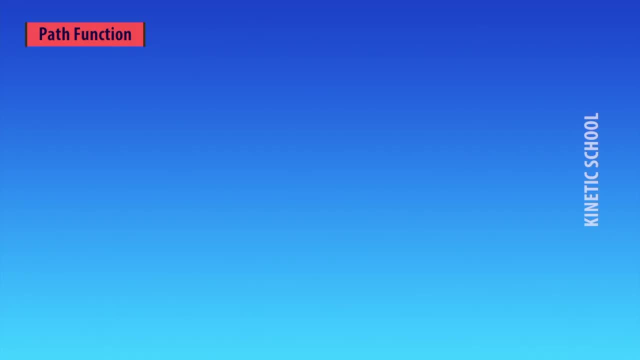 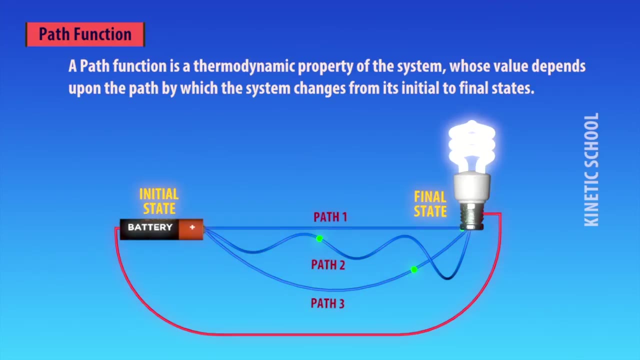 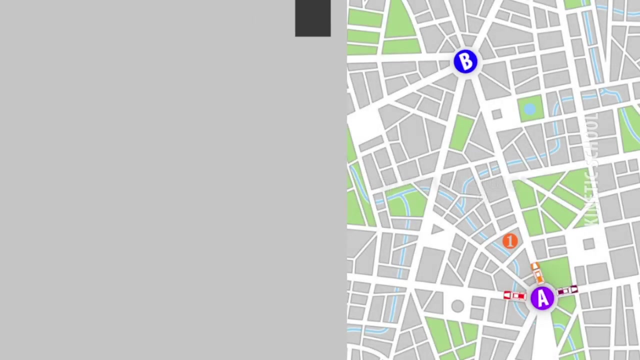 volume, pressure, internal energy, enthalpy, entropy are the state functions, Path function. A path function is a thermodynamic property of the system whose value depends upon the path by which the system changes from its initial to final states. Let's see an explanation.